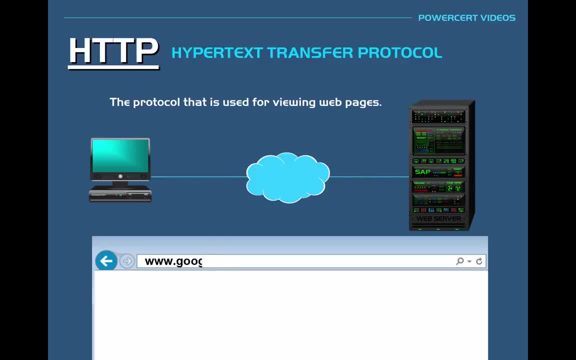 So when you type in a web address like googlecom, you'll notice that HTTP is automatically added at the beginning of the web address, And this indicates that you are now using HTTP to retrieve this web page. Now, in standard HTTP, all the information is sent in clear text. 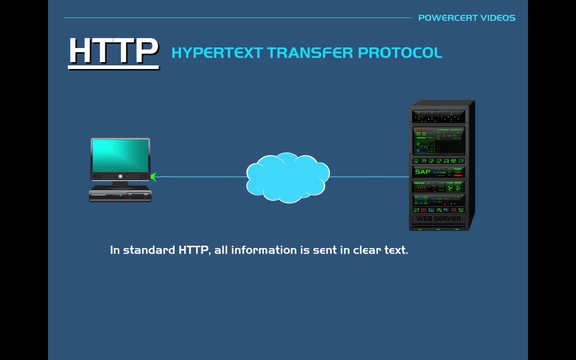 So all the information that is exchanged between your computer and that web server, which includes any text that you type on that website, that information is transferred over the public internet And because it's transferred in clear text, it's vulnerable to anybody who wants it, such as hackers. 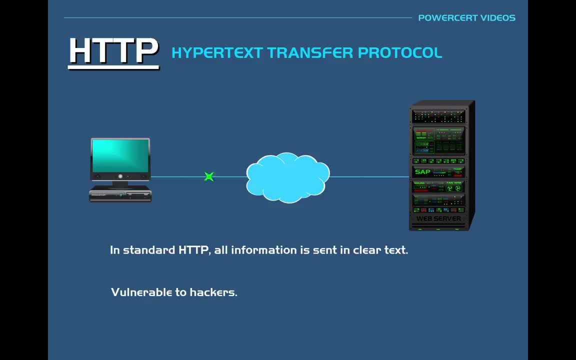 Now, normally this would not be a big deal if you were just browsing regular websites and no sensitive data such as passwords or credit card information are being used, But if you were to type in personal, sensitive data like your name, address, phone number. 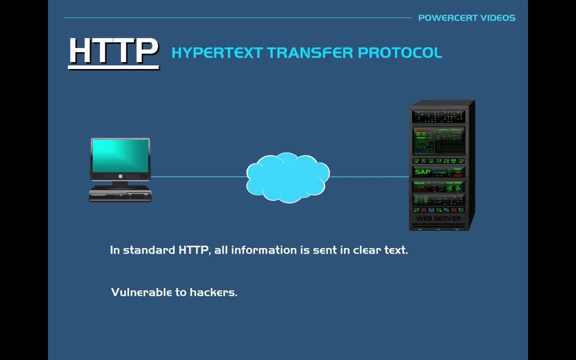 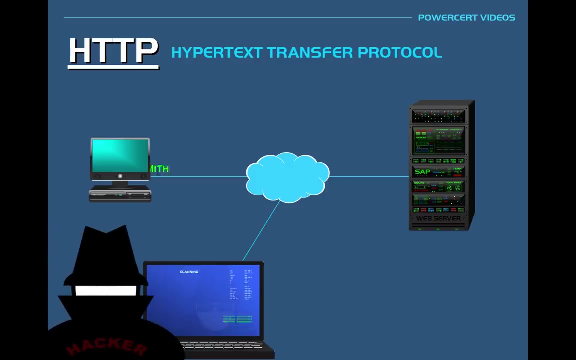 passwords or credit card information. that sensitive data goes from your computer and then it has to transfer to your computer And then it has to travel across the public internet to get to that web server. And this makes your data vulnerable because a hacker that's somewhere on the internet can listen in as that data is being transferred and steal your information. 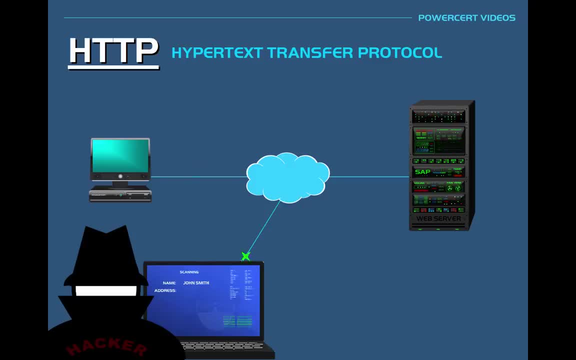 So, as you can see, this hacker is stealing personal information, as it's traveling over the internet. So he has a name, phone number, address, credit card numbers and so on. So this is a problem as far as security is concerned. 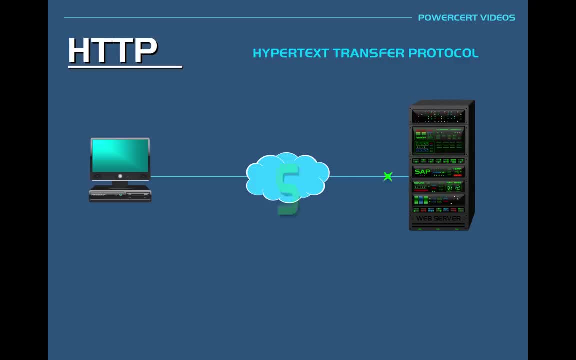 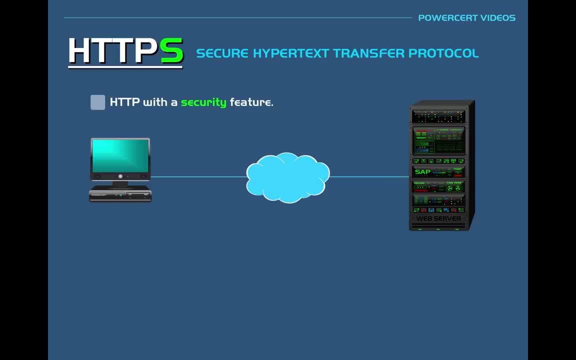 And this is HTTP with a security feature. Secure HTTP encrypts the data that is being retrieved by HTTP. It ensures that all the data that's being transferred over the internet between computers and servers is secure by making the data impossible to read, and it does this by using encryption algorithms to scramble the data that's being transferred. So for 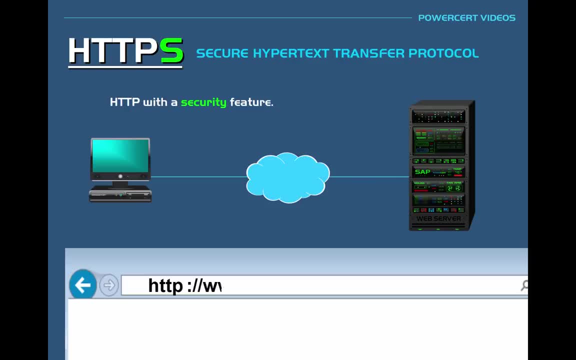 example, if you were to go to a website that requires you to enter personal information, such as passwords or credit card numbers, you will notice that an S will be added to the HTTP in the web address, And this S indicates that you are now using secure HTTP and have entered a secure 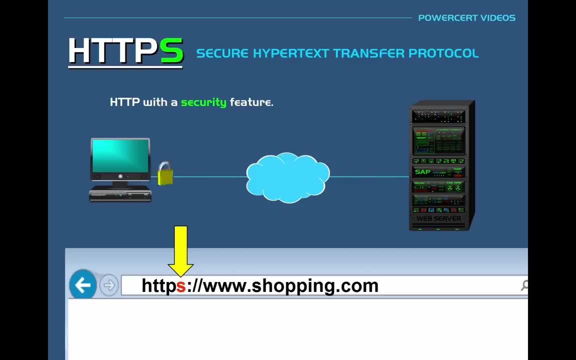 website where sensitive data is going to be passed and that data is going to be protected. And, in addition to the S being added, a lot of web browsers will also show a padlock symbol in the address bar to indicate that secure HTTP is being used. So, by using secure HTTP, all the data which 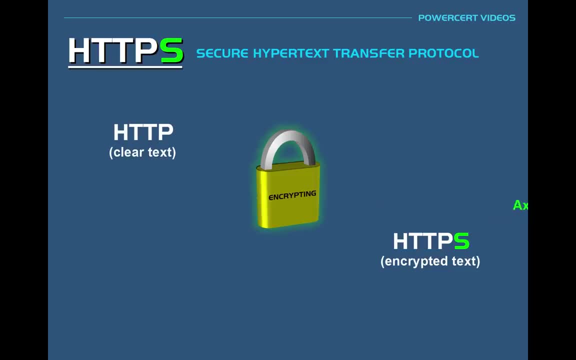 includes. anything that you type is no longer sent in clear text. it's scrambled in an unreadable form and is then sent to the web. So if you were to go to a website that requires you to enter personal information as it travels across the internet. So if a hacker were to try and steal your information, he would 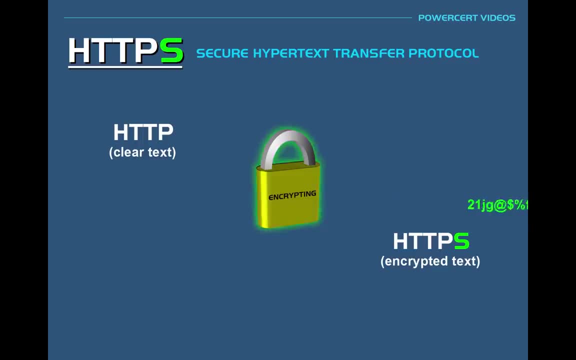 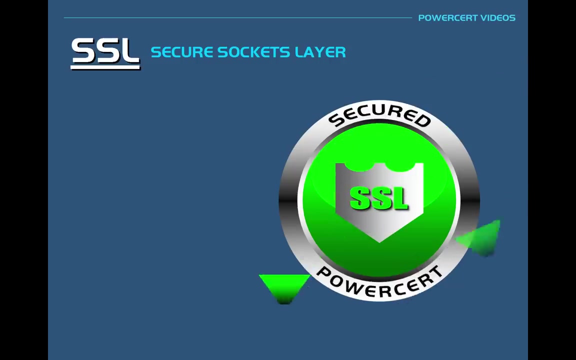 get a bunch of meaningless data because the data is encrypted and the hacker would not be able to crack the encryption to unscramble the data. Now, secure HTTP protects the data by using one of two protocols, and one of these protocols is SSL. SSL, or secure sockets layer, is a protocol that's used. 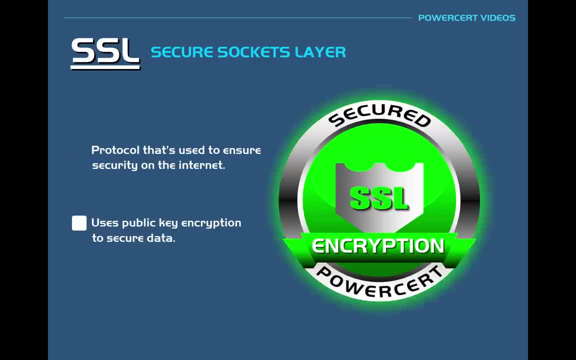 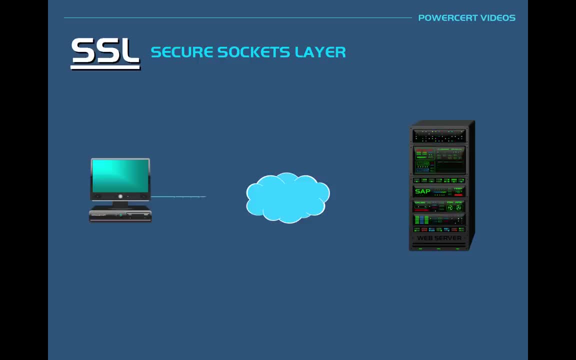 to ensure security on the internet. It uses public key encryption to secure data. So basically, this is how SSL works. So when a computer connects to a website that's using SSL, the computer's web browser will ask the website to identify itself. Then the web server will send the computer. 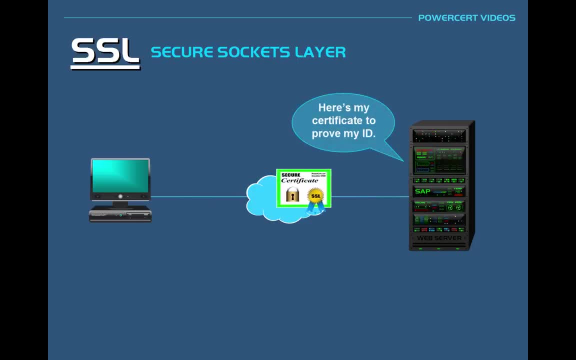 a copy of its SSL certificate. An SSL certificate is a small digital certificate that is used to authenticate the identity of a website. Basically, it's used to let your computer know that the website you're visiting is trustworthy, So then the computer's browser will check to make sure. 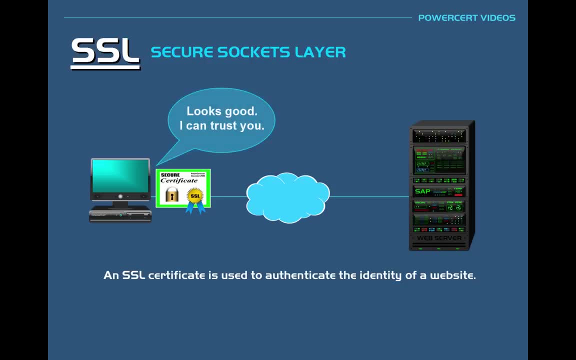 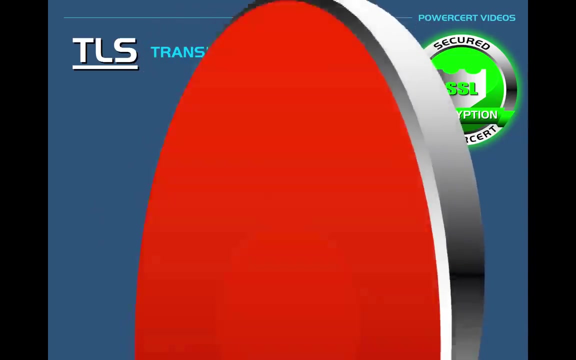 that it trusts the certificate and if it does, it will send a message to the web server. Then, after, the web server will respond back with an acknowledgement so an SSL session can proceed. Then, after all these steps are complete, encrypted data can now be exchanged between your computer and the web server, And the other protocol that secure HTTP.